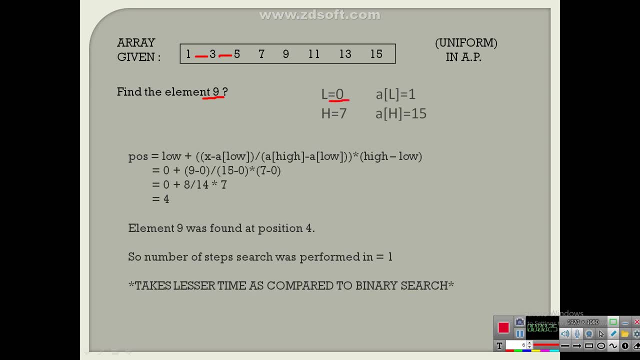 The lowest element will always be zero. Highest element will be seven. over here, because we are having eight elements, The value stored at the lowest index is one and that of the highest index is fifteen. Now we have to first understand that. which index should we search first? 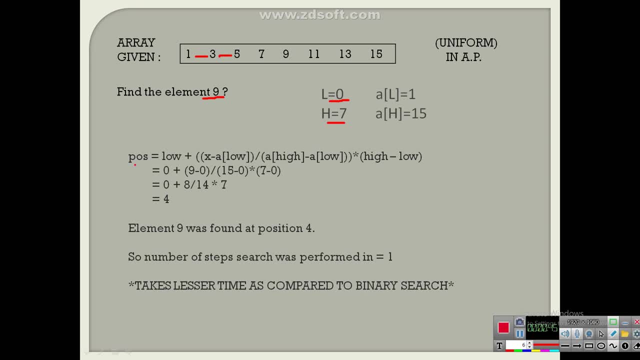 And whatever index will be searched first will get stored in this variable position. Now this is calculated using this formula. Okay, So after performing the calculation, the position will get the index where we should look first. So we got the answer four. 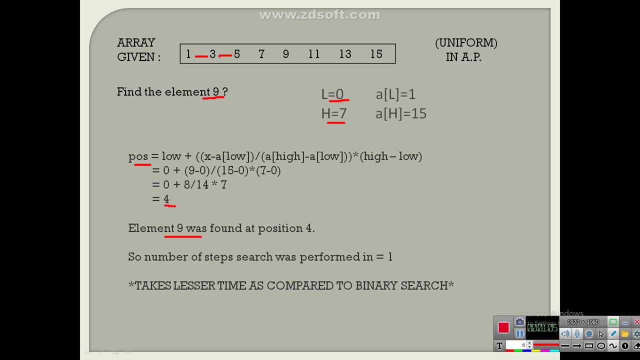 So we can say that the element nine was found at position four. Now, since this array was uniformly distributed, the number of steps required to perform was only one, And it clearly takes less time than the binary search. So, on looking on the fourth index, we have got our element nine in only a single step. 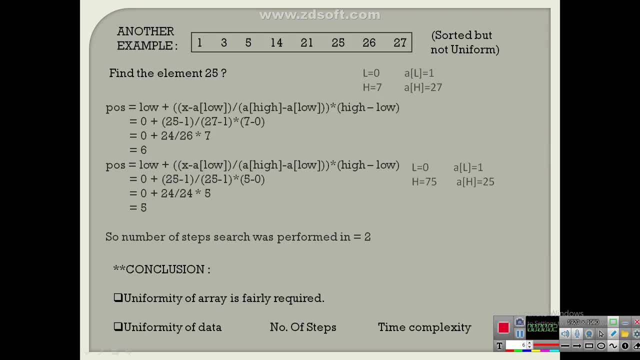 Okay, Coming to the next example, where the uniformity of elements is less as compared to the previous array. Here we can see that the distance, sorry the gap between first element and the second element is two, Then here it is nine, and so on. 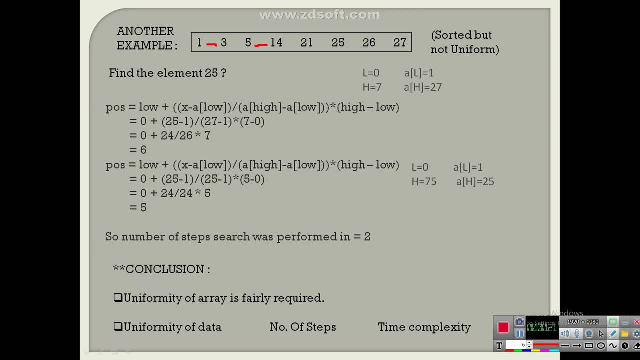 So we can say that this array is sorted but not uniform. Here we are being asked to find this element twenty-five. Okay, So we have already written the value, the initial values of the lowest index, highest index and the values stored in this index. 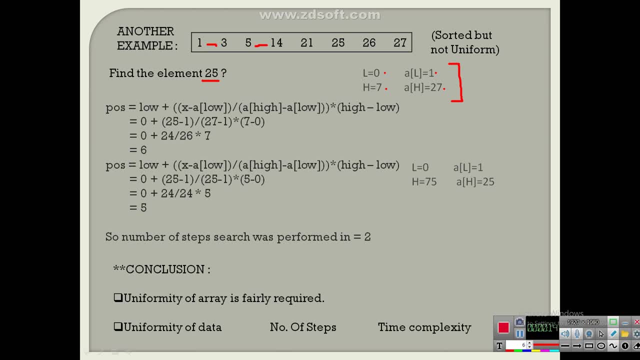 Okay, The element to be found out is our x, here twenty-five, And we are using these values here to find the first index where we are supposed to look for the element twenty-five Here, after performing the calculation, we will get a value six point something, but we will only take six because the index is never a float value. 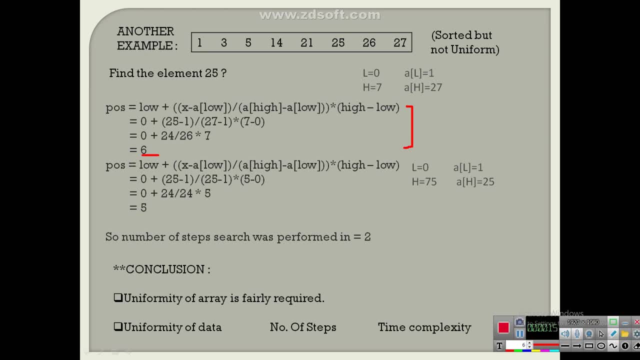 It is always an integer, So we are considering only the floor value. Now we have got the first index as six, So we will look for the element twenty-five in the sixth index. Now if we see in the array in the sixth index we already have element twenty-six. 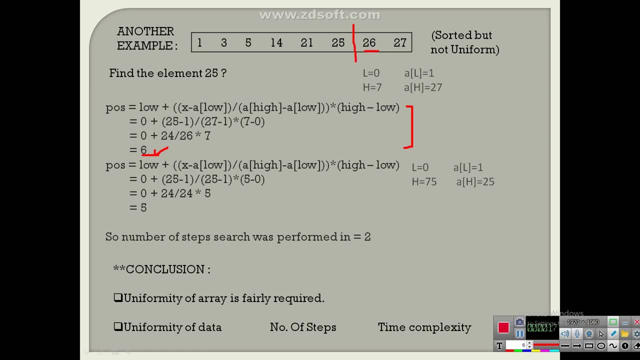 Now what we will do is we will divide this array into two parts And, since this twenty-five is obviously less than twenty-six, we will take this left half of the array and we will search for twenty-five. Now, since we have shortened our array, it only contains six elements. 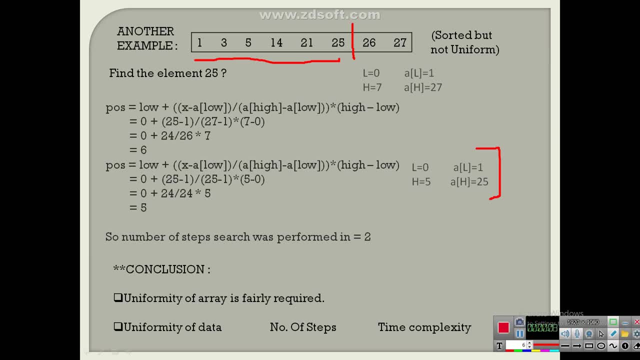 So we will reassign the indices value. Only the highest index will change And the element contained in it will also change. And now we will use these values to again find the new index for finding the element twenty-five, which might contain the element twenty-five. 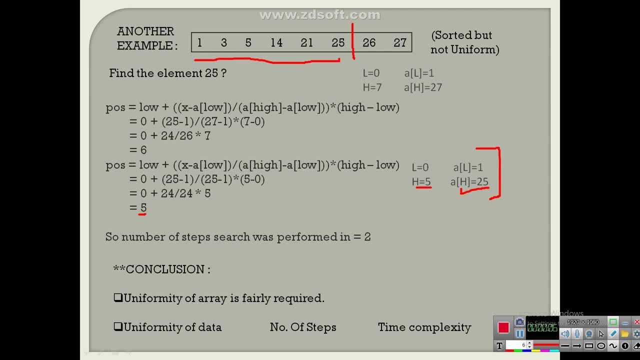 So after putting the new values, we get exact five over here as our answer. So we can say that the element twenty-five was found at the fifth index, which is true. So our element twenty-five was found at the fifth index. 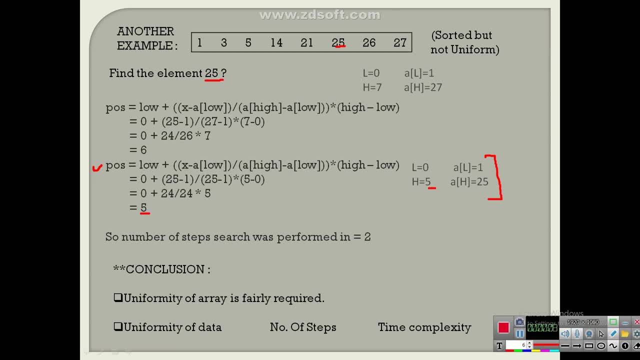 Fine. Now we can say that the number of steps required to perform this search was two, which means that if we are taking more than one step to perform the search, we can say that the array is not uniform. That is why the search is taking more time. 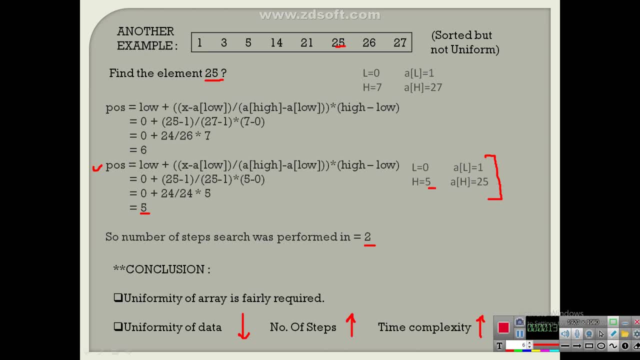 So if the uniformity of data decreases, then the number of steps required to perform the search increases and so does the time complexity. While for the binary search the time complexity is fixed, this time complexity of interpolation search solely depends on the uniformity. 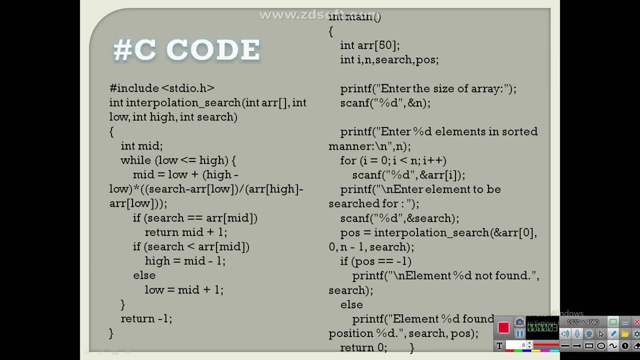 So that was the algorithm for interpolation search. This is the required C code to perform this search. Here I have created a function called interpolation search, as you can see, And this will carry out the calculation. Then in the main function I have asked the user to enter the size and the element stored in the array. 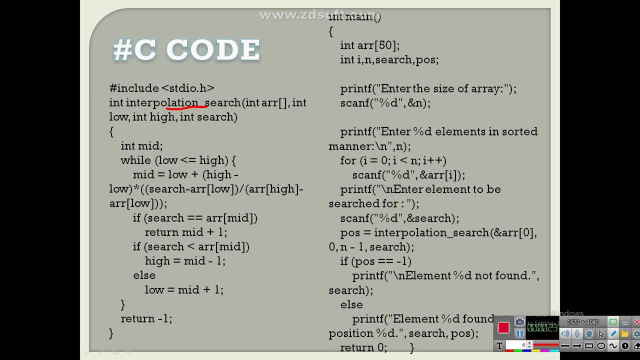 And then I have performed this search. If the element was present in the array, it will show its specified position. Otherwise, it will write that this particular element was not found. So yeah, this is the interpolation search, how we can perform this search in the C code.